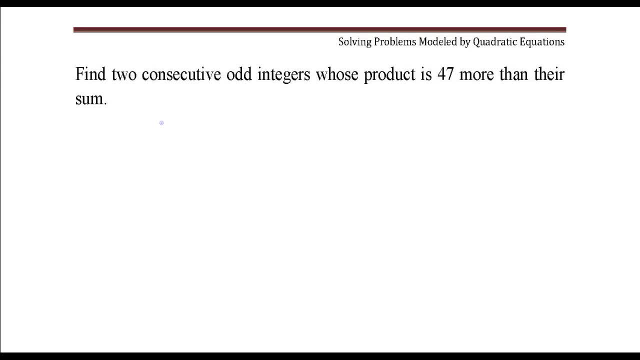 Let's let the first odd integer be x and then the next consecutive odd integer would be x plus 2.. So the product of these two numbers is 47 more than their sum. So the product of those two integers is- that's the equal sign- 47 more than the sum of those two integers: x plus x plus 2.. 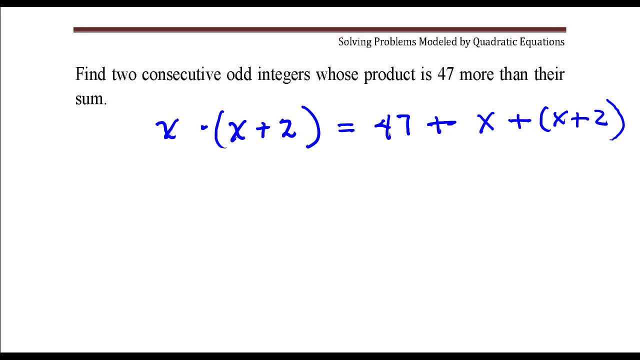 So all we need to do is solve this equation. I'll distribute here first. So this is going to be an x plus 2.. x squared plus 2x is 49 plus 2x. If I subtract 2x from both sides, these will become 0.. I'll be left with x squared is equal to 49.. 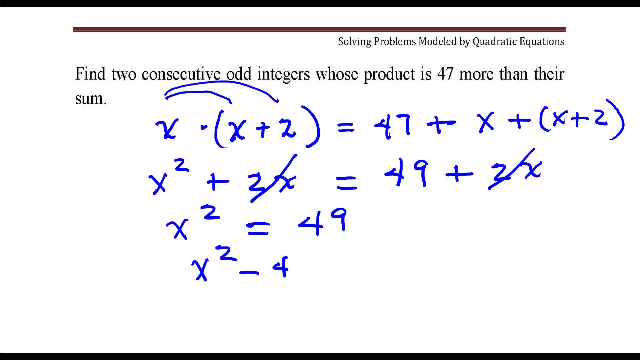 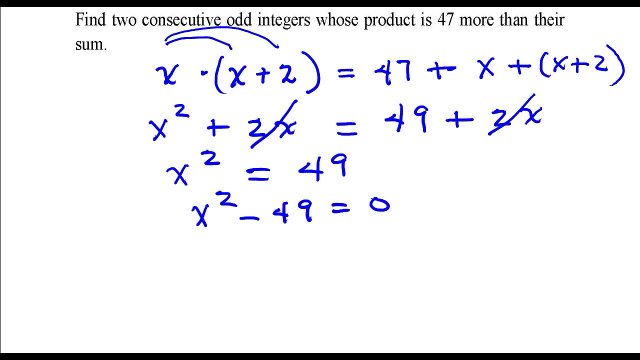 Subtract 49 from both sides Gives me a binomial that is quadratic. I can factor this: This is a difference of two squares. Factor this into a product of two binomials. Set each factor equal to 0.. Solve each equation. So x is negative 7 and x is positive 7.. 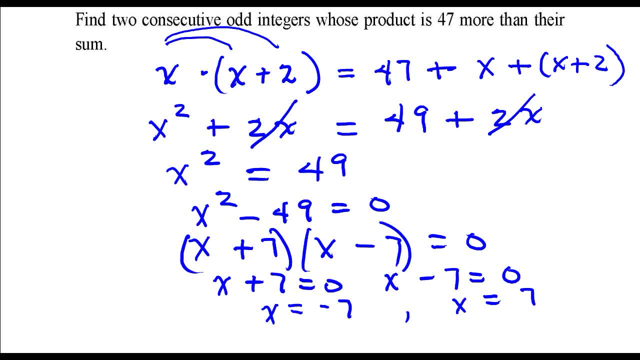 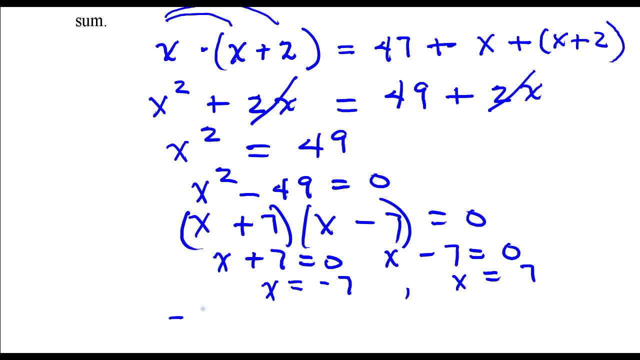 So we're looking for two consecutive odd integers. So let's take this first answer, negative 7, first. So if this is the first odd integer, then the next consecutive odd integer would be a negative 5.. And for this answer, if 7 is the first integer, then its consecutive integer would be a 9.. 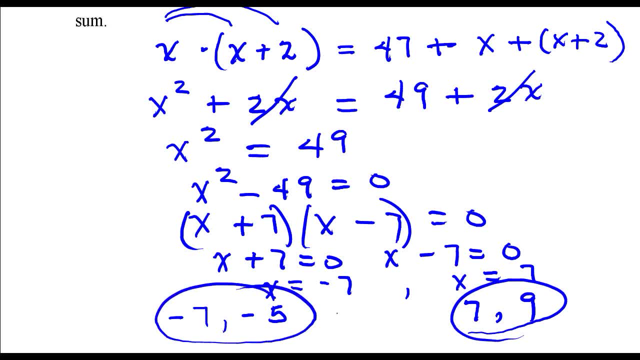 You can look at this as an obvious principle in a lesson in the past. All right, so for the correct answer, what we want to do is similar to the initial factor. We'll use this as an incomplete factor in this section. we want to use an infinite number. So we have this gy balcony parameter. I just want to make sure I'm able to calculate over a total of hear. What I'm going to say is 2 over 4.. I'm going to write this as a possible answer. Here's the answer in the column: